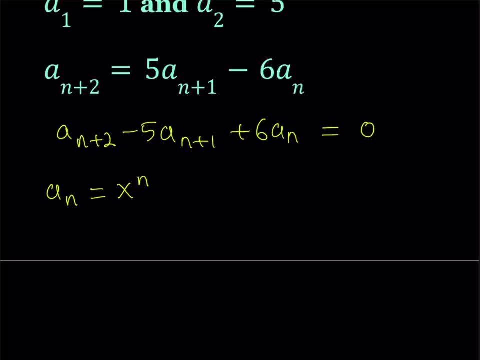 The sequence, hopefully also using the initial conditions. So now, since that's a n, I can just write a n plus 2 as x to the power n plus 2 minus 5 times x to the power n plus 1 plus 6 times x to. 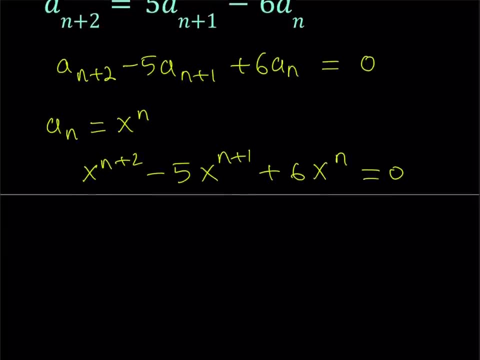 the power n equals 0.. So this is going to give us an equation, but let's go ahead and factor out x to the power n first. Since this is x to the power n times x squared, I get x squared minus 5x plus. 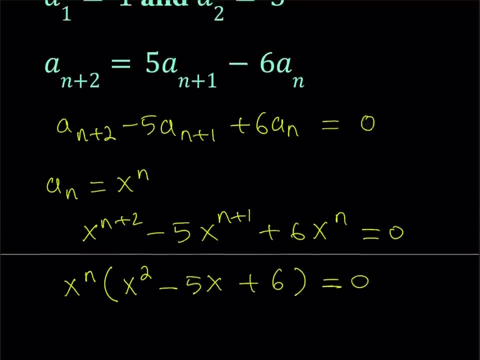 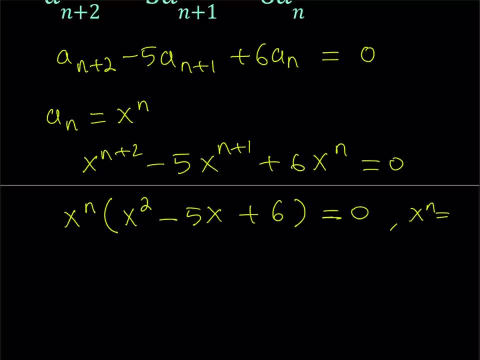 6 equals 0.. Now, given the sequence, the terms, the first two terms and the rule, we know that x to the power n does not equal 0. Therefore, from here- and it's not going to be equal to 0 all the time, obviously for all x values- So from here we get that x squared minus 5x plus 6 is equal to 0. Now, 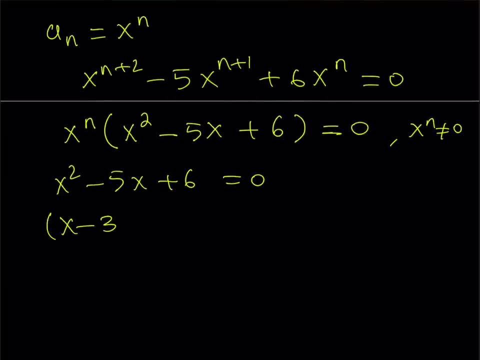 we can factor this equation easily as: x minus 3 times x minus 2 equals 0, and from here we can get the x values as: x to the power n times x to the power n plus 2 times x to the power n equals 0.. 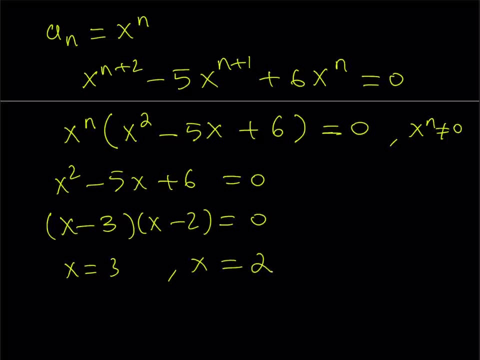 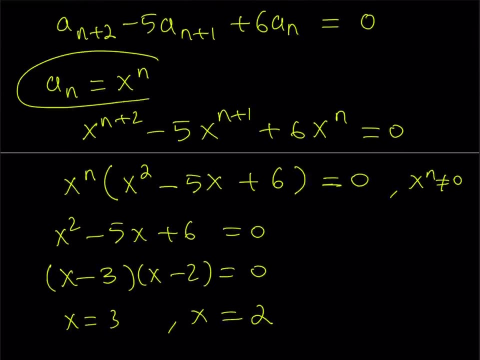 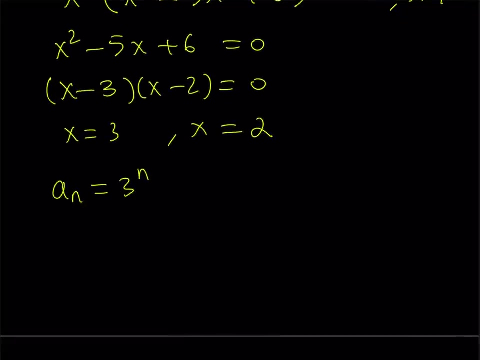 So we get a quadratic equation which is a characteristic equation again. So this means we we assume that a n could be written as x to the power n and we found these two values. So this means that a n equals 3 to the power n should satisfy the sequence If you plug it in. 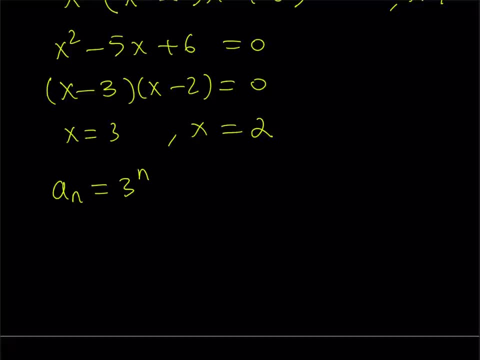 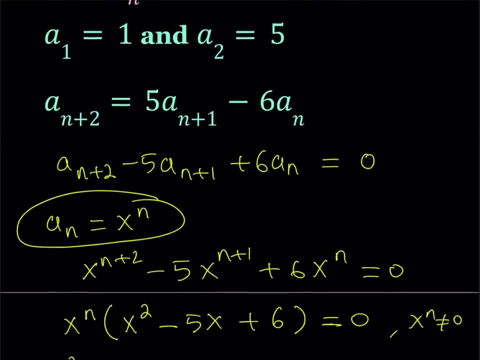 you're going to notice that it does. and the same thing goes for 2 to the power n. But we're going to also have to consider the initial conditions here. We're given that a 1 is equal to 1 and a 2 is equal to 5.. If we just assume that a n is equal to 3 to the power n, for 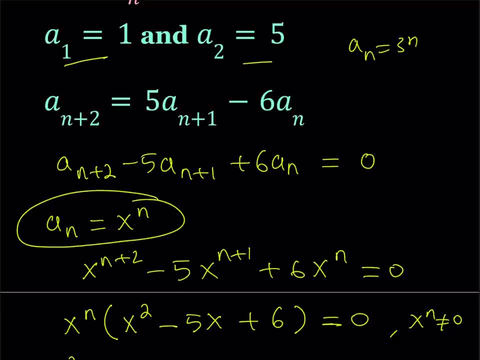 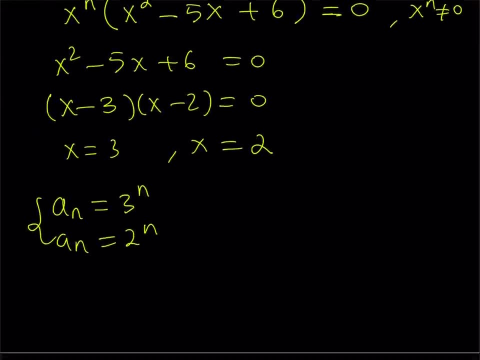 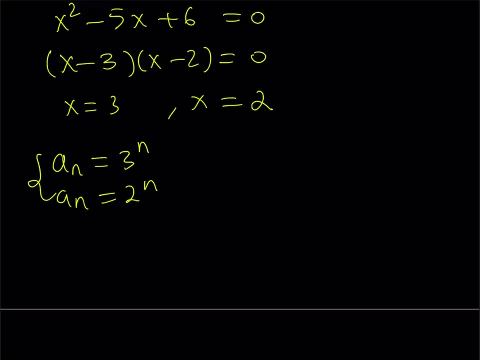 example, then these are not going to be satisfied, nor are they going to be satisfied with 2 to the power n. So we have to do something else. So we're going to put these together. Obviously, if 3 to the power n and 2 to the power n are both solutions for this recursive sequence, then their sum is: 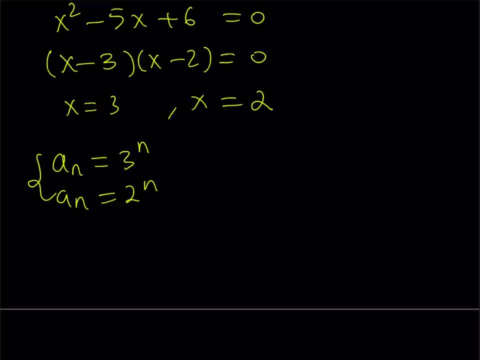 also a solution. their difference is also a solution and in general, any linear combination of these two will also be a solution. So we're going to write the general solution for a n as a linear combination of 3 to the power n and 2 to the power n, And this is what it looks like. 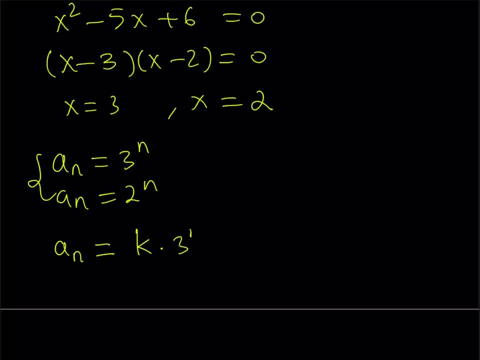 a n equals k times 3 to the power n plus m times 2 to the power n. Now here, k and m are real numbers, so they can be pretty much any real number and we're going to find those numbers Using what The initial conditions. So let's go ahead and do that. So we got the form for a n. now let's go ahead. 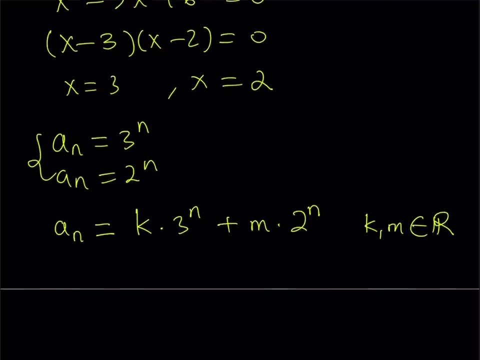 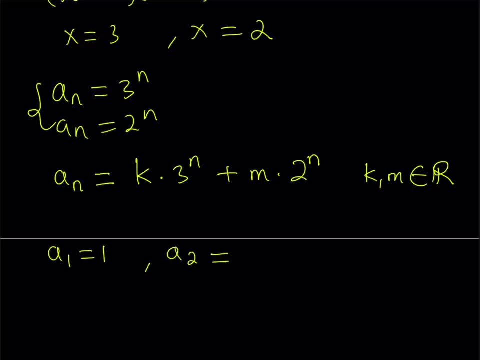 and use the initial condition. What are the initial conditions? Well, we're given that a 1 is equal to 1.. So we know that a 1 is equal to 1 and a 2 is equal to 5 from the sequence, because our 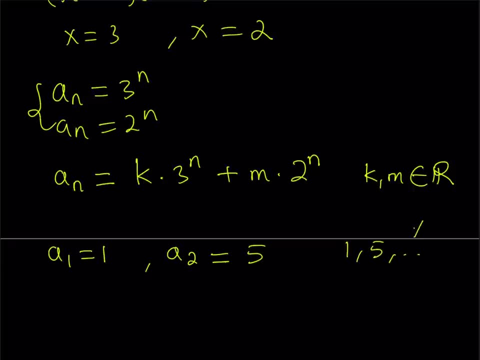 sequence goes like this: Now we can also evaluate a 3 here by way of substitution, but that's not needed, because all we need is two equations. We have two unknowns And we can just use a 1 and a 2 here. but if you want to verify your result, obviously you can also. 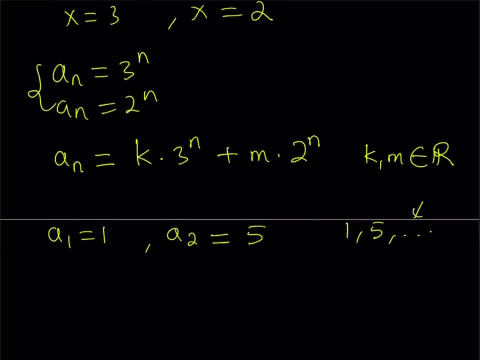 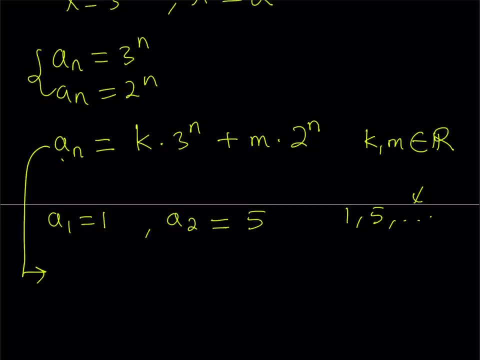 use a 3 or any other term in this case. Okay, so let's go ahead and replace n with 1 here, in this sequence That's going to give me. if you replace n with 1, you get 3k plus 2m equals a 1, which is 1. 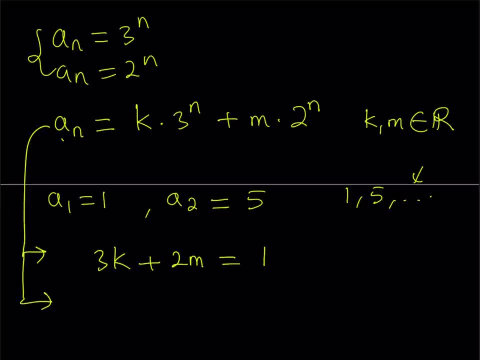 and then if you replace n with 2, then you're going to be getting. so this is n equals 1.. And this is 4 and equals 2.. If you replace n with 2, then you get 3 to the second power, which is 9.. 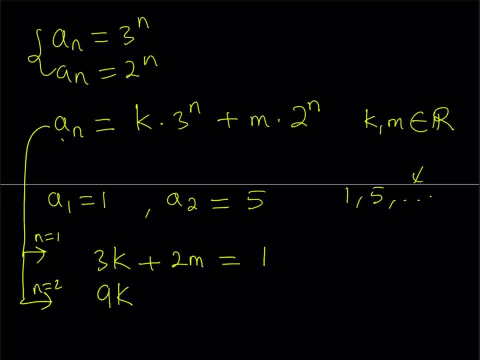 So that gives me 9k. 2 to the second power equals 4.. So that gives me 4m, and this is equal to a 2, which is 5.. Great, So now I got a system of two equations. This is linear and easily solvable. 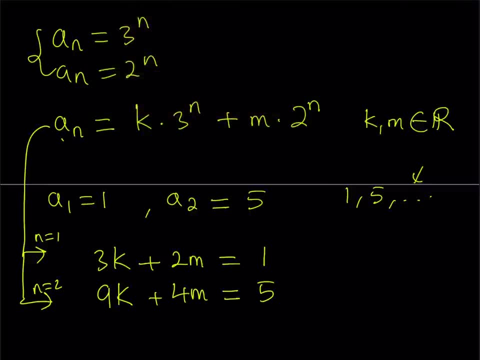 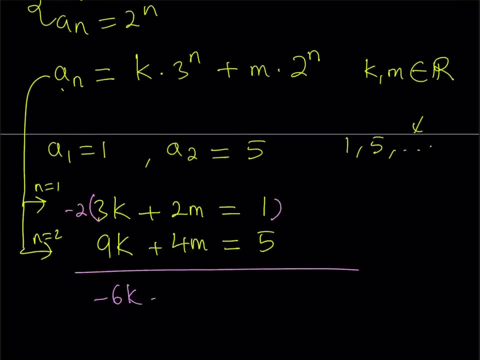 So let's go ahead and solve this system. I'm going to eliminate m, So let's multiply the first equation by negative 2.. And this gives us negative 6k minus 4m equals negative 2.. And the second equation stays, the. 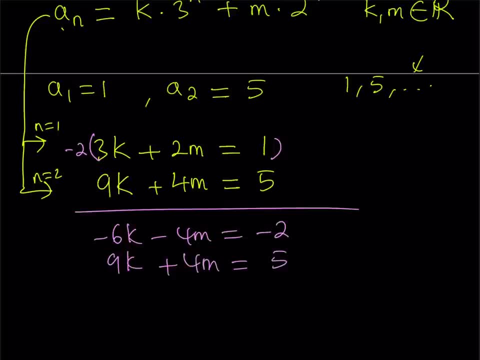 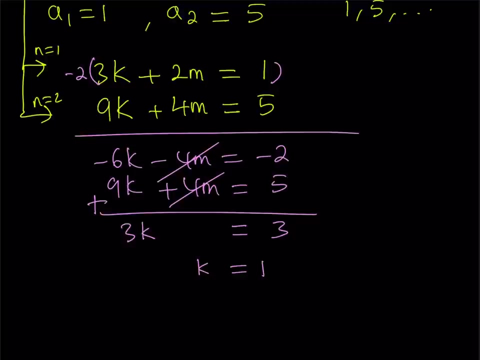 same. And now I'm going to add these: to eliminate m, And this gives me 9k minus 6k, which is 3k equals 3. And from here I get k equals 1.. Great By way of substitution, if you replace, for example: